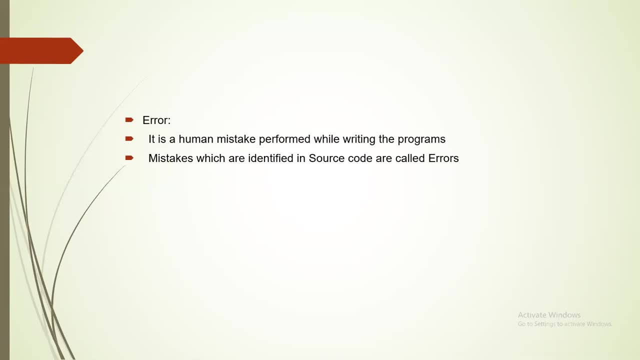 code are called errors. Mistakes which are identified in source code is called errors, For example, logical errors and syntax errors, these things. But as a tester you are not going to identify this kind of errors because we are not going to test the source code. Second, one defect. Defect means it is a deviation. 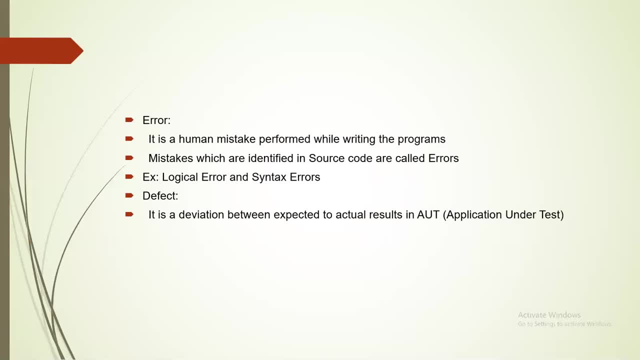 between expected to actual results in AUT, application under test or system under test. also we are going to call Defect can also called as an issue or incident or fault. Defect can also called as an issue or incident or fault. Defect can also called as an issue or incident or fault. 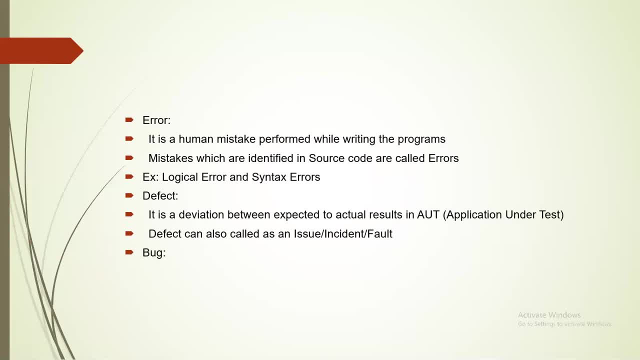 Bug Whenever defects were identified. as a test engineer, we are not the responsible to solve the defects. What we have to do, We need to intimate to the developers. When we report it to the developers, developers will do the review on the defects to confirm those are valid defects or not. If those defects are, 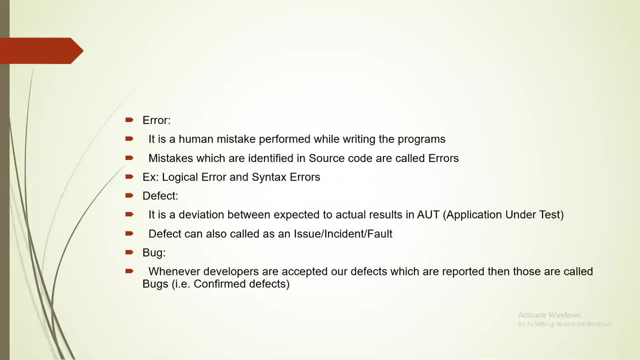 valid, then those are called bugs. That means whenever developers are accepted our defects which are reported, then those are called bugs. That means confirmed defects- Failure. Failure means whenever defects are reaching to the end user, then it is called failure software Due to poor performance of testing team. So testing team said that 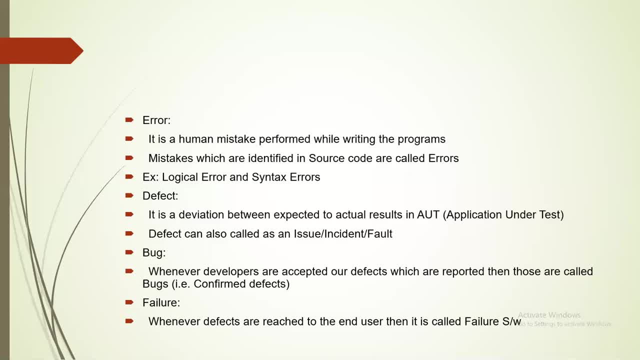 everything is working fine based on your rewards project delivered to the customer. But when you are using software- customer finding the problem, then it is called failure software we are going to call. There is a difference among the error defect bug and failure Defect. 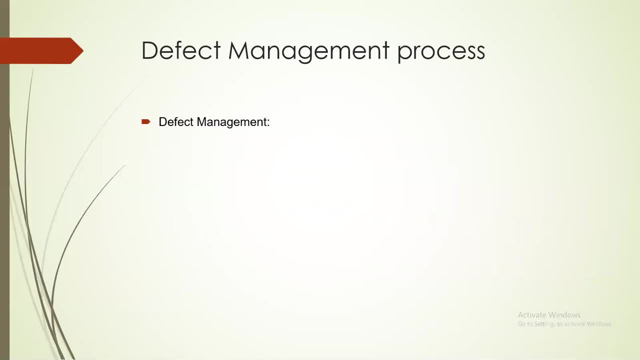 management process. now we are going to discuss What is defect management. Defect management is a process of identification of defects, reporting, tracking and closing the defects for a project is called defect management. Defect management is a process of identification of defect, reporting, and tracking and closing the defects for a project is called defect. 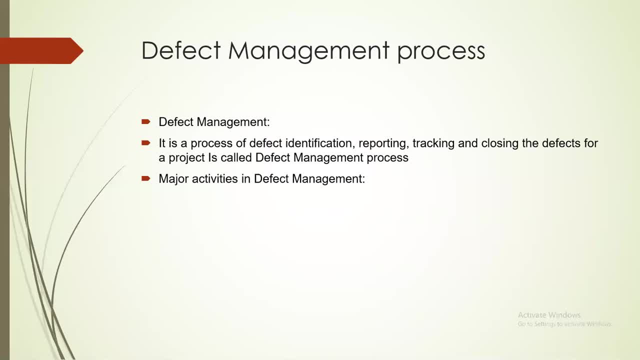 management process. What are the major activities in defect management process? First one is Defect identification. Second one Defect reporting. Third one Defect tracking. Fourth one Defect re testing. Fifth one Defect closing. eleventh one Defect Detector. On third one: the other one is Defectと Put, but here, if not, exactly what type will come out? this is linked: If it is a polybutyl bawling from an on one device, then in this southwest department is containing different defects, another below each one will have a prevail or not, And more likely is this the actually getting the GDP sitting below this究 device. because of this is now in the process staff solutions available which you may. 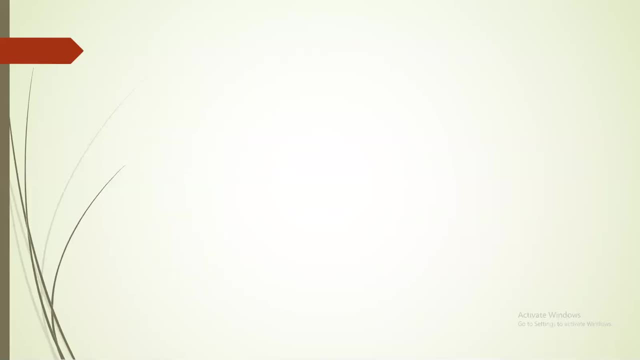 activities during defect management process one by one place. we are going to see detailed defect identification as we know that, as a tester, when we are going to identify defects during test cases preparation are while doing the review in the requirement office, no, at the time of test cases execution, whenever we 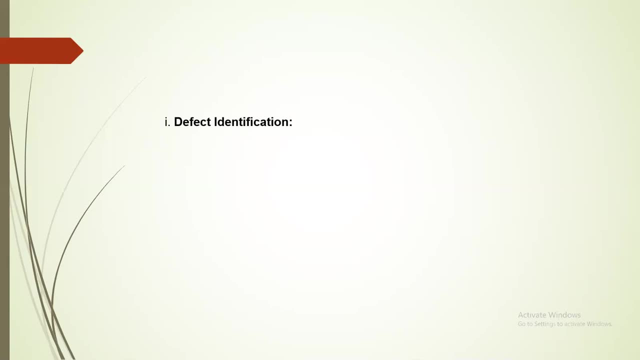 identify deviation between expected to the actual results that we are going to defeat. the different can also called as an issue or incident, or fault is a well executing test cases. whenever we identify deviation between expected to actual results in a UT, is called different our issue or incident or fault. 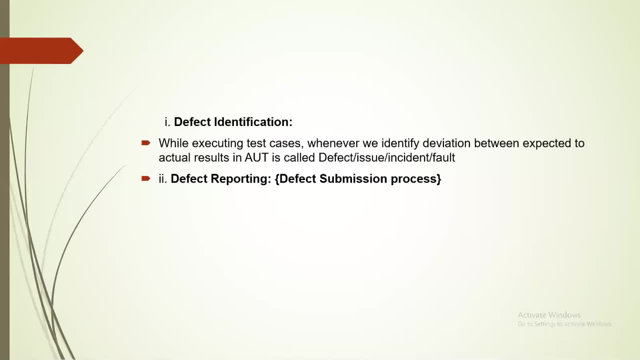 second one, defect reporting. so the fact submission process also are going to call. what is the meaning of the? notifying about the defects to developers is called defect reporting. notifying about the defects to developers is called defect reporting. what are the guidelines to lock the defects? every tester should know. it is the moment when testers identify the defect. in current project we are 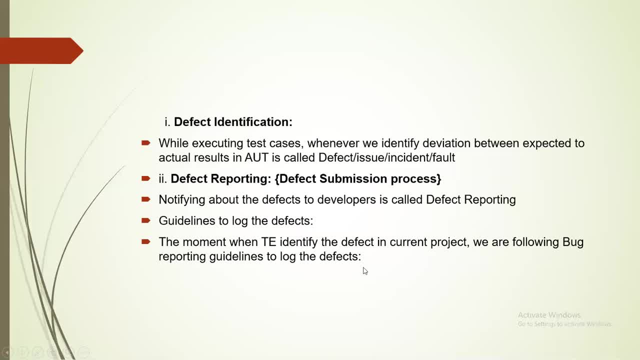 following bug reporting guidelines to lock the defects. what are the guidelines? the very first thing whenever you identify defects. so any defect you identified once again we have to recheck the same functionality in application to confirm that defect will occur every time or part. that means the defect is the vehicle is good or not. the first thing then try to check the same functionality. 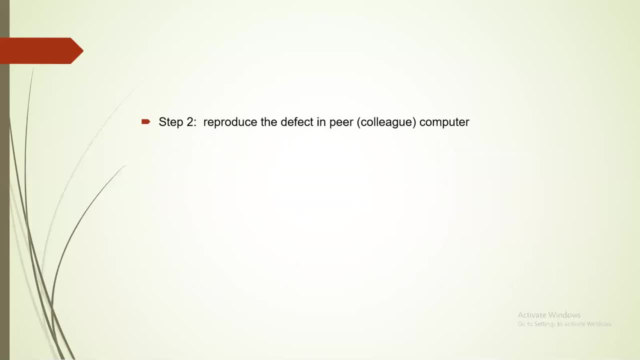 in your colleague computer because environment in that environment is going to be so difficult rise or not. check the defect in database for duplication. same defect may be already identified by some test engineer which is already reported. you need to confirm it is. look into the so defect database. step four: drop the bug. drop the bug is prepare the defect profile. 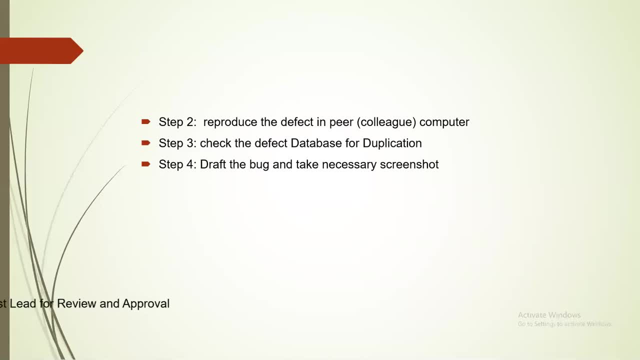 and take necessary screenshot. step five: send the email to test lead for review and approval of your defect which you identified. then step six: once bug is approved by test lead, then test engineer login into defect tracking tool and submit the bug to development lead. but whatever defect you are reporting, the defect first time you identified should give the status as: 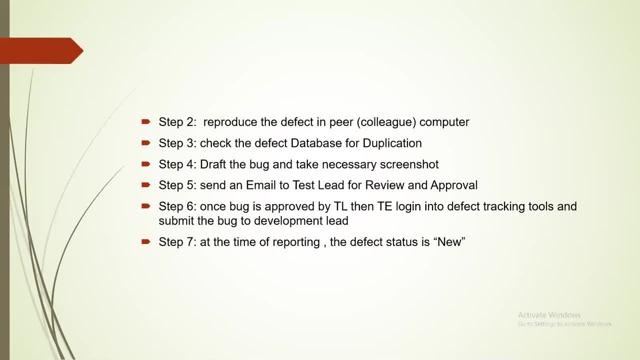 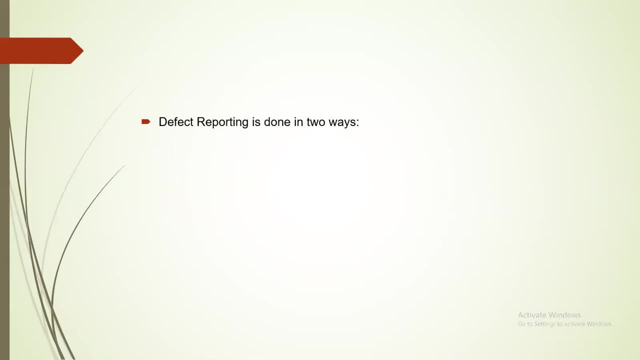 new. these are the seven steps you have to follow. but to lock the defects, defect reporting is done in two ways. difference in the organization it may varies. one is manually, the other one is automation. manually- what is that? manually copy the defect template from file server or vss. every organization will maintain the one defect. 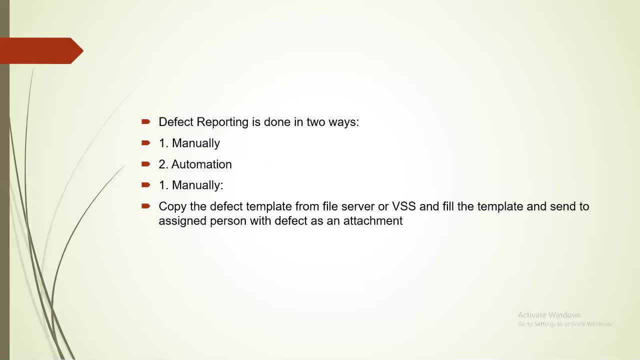 template. so the template will be given to you, templates which are some pretty different component or skeleton of the document. so where, from where we are going to get they will: file server or vss visual sources. so this is the common repository will be there. so in my playlist i 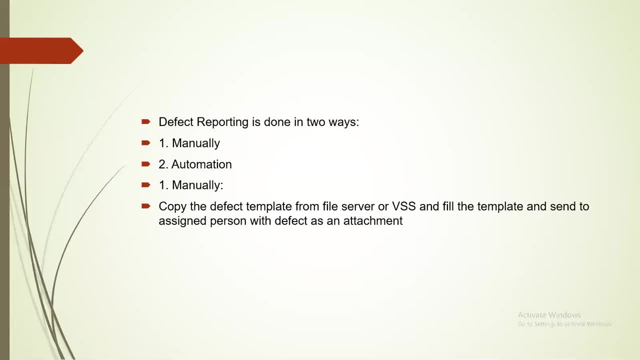 provided the vss visual source if also, if you want to watch, you can watch. it is around one hour, it's complete spaces. so and fill the template sent to assign the person with the defect as an attachment. other possibility: automation. we can use some third-party tools for defect reporting purpose. we have the various tools like 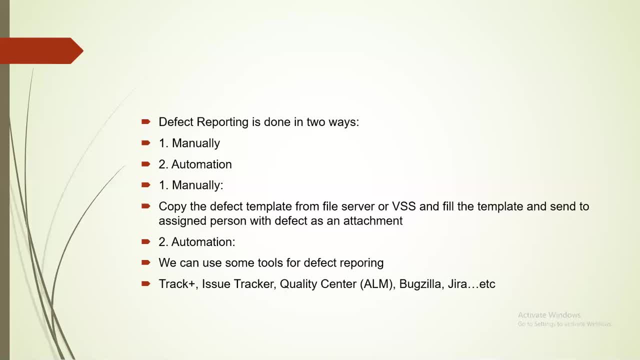 trackless issue tracker, quality center. now it is called a limb application lifecycle management bugzilla, Jira, clear twist PR tracker like this. various tools are available. some companies are going to use their own tools also, like article company will use the OPM article test management tool. okay, like that. so 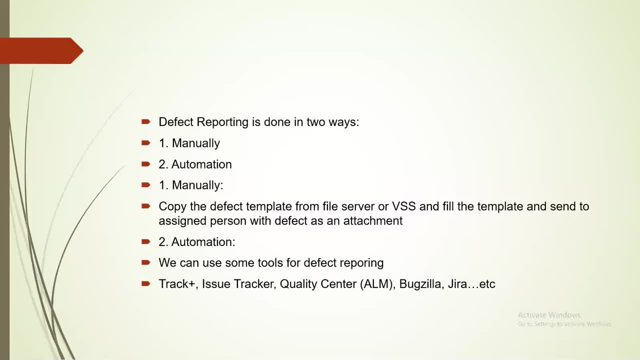 different tools are available and this are very simple tools. it is like how we are going to use Gmail to send me similar way. it is thought one in defective engine process. first, one will be infantry, different education. second, one different reporting, not one defect tracking. what is this? 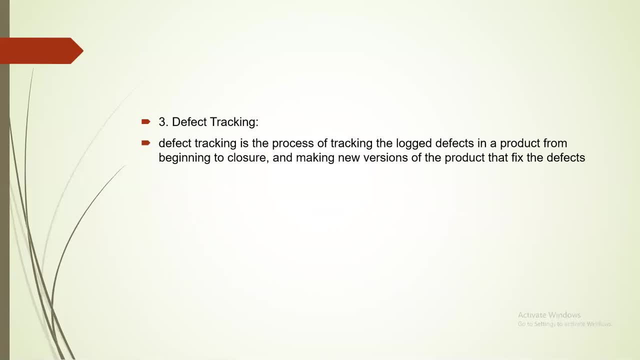 defect tracking. effect tracking is a process of tracking the local defects in a product from beginning to closer and making new versions of the product that fix the defects. so we have to. what are the defects identified? or opposite accident, which is state those are fixed on. so resolved properly or not? history is confirmed on like center. 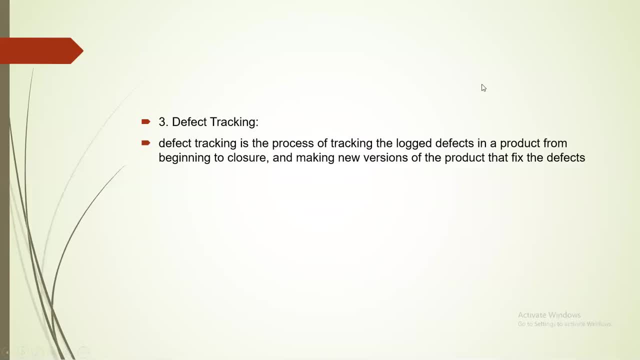 process we are going to track. that is called defect tracking. we are going to, for the fourth one, different retesting. as you know, the retesting is where we are going for all modified ability, so to check bugs are resolved on, so not all the different which are reported. if test lead will assign the fixed defects for. 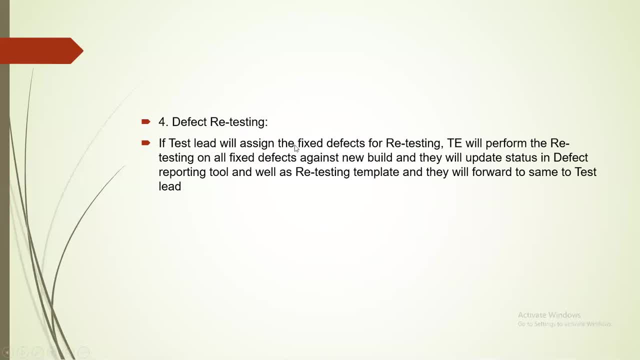 retesting fixed defects. which defects are? the state circuits, those type of defects test you will perform the retesting on all fixed defects again is new build and they will update status in defect report to as well as retesting template and they will forward to same to test new. they follow to test new. that defect, retesting if the one defect closer. so once a defect has been a result and a verified, that defect is changed status as closed. so once we satisfied about the defect resolved, we give this status as closed. if not, we have sent a notice to the development development team to check the defect. 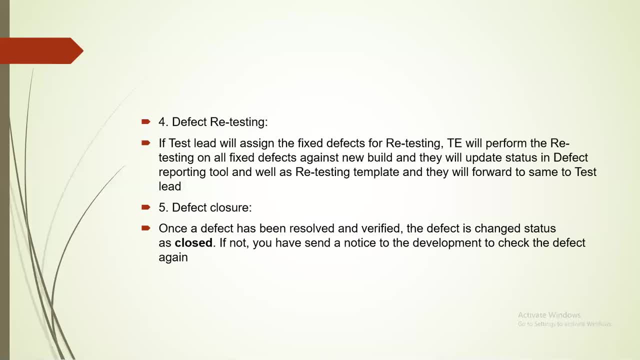 again by providing statuses and reopen. reopen in the status for the next session. I'm going to explain the bug: life cycle. what are the different kind of status are going to given? so what is what life cycle? these things are going to understand it in the next session. but